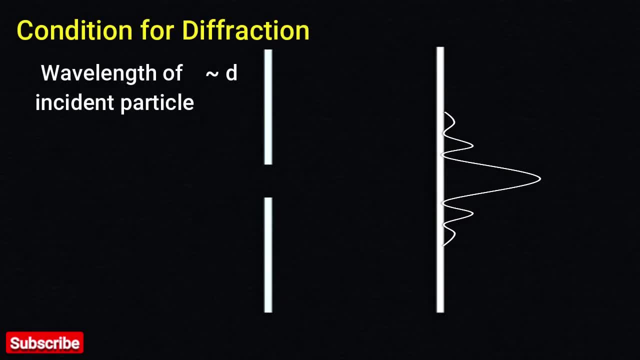 when we have wavelength of the incident particle comparable to the slit width. And for the sake of simplicity, let we only confined to the central maxima. This maxima and minima's are dependent on the part difference. So let's first calculate the part difference. Suppose there are two electrons: 1., 2., 3., 4., 5., 6., 7., 8., 9., 10., 11., 12., 13., 14., 15.. 16., 17., 18., 19., 20., 21., 22., 23., 24., 25., 26., 27., 28., 29., 30., 31., 31.. 32. 33., 34., 34., 35., 36., 36., 37., 37., 38., 38., 38., 38., 38., 38., 39., 39.. 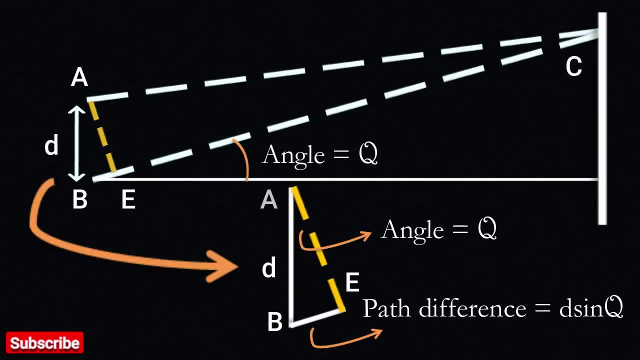 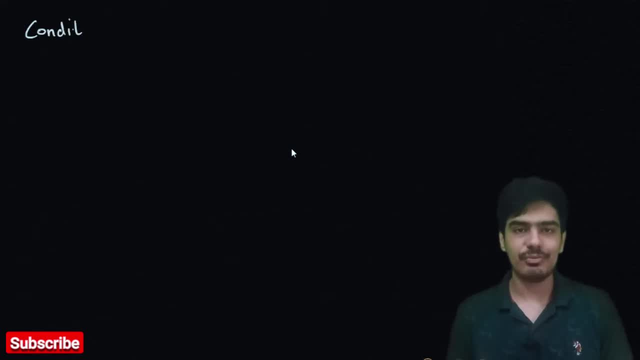 39.. 39.. So this part difference is equal to d sine theta, where d is the slit width. So now we have our part difference. Now let's take the condition of minima, which is part difference is equal to n lambda, where 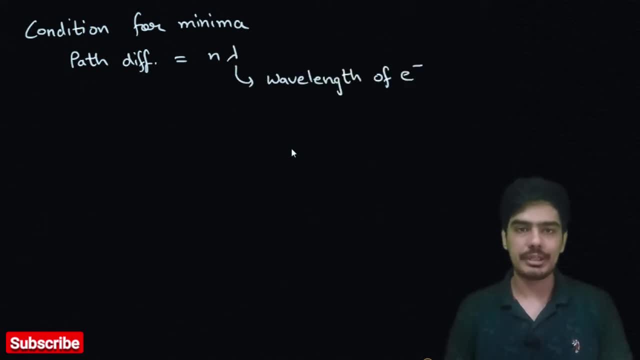 lambda is the wavelength of the wave corresponding to the electron, and n is the order of the minima, and we have part difference as d sine theta. So our equation becomes: d sine theta is equal to n lambda. So for the simplicity, let us confine ourselves to the central maxima means. we are only taking. 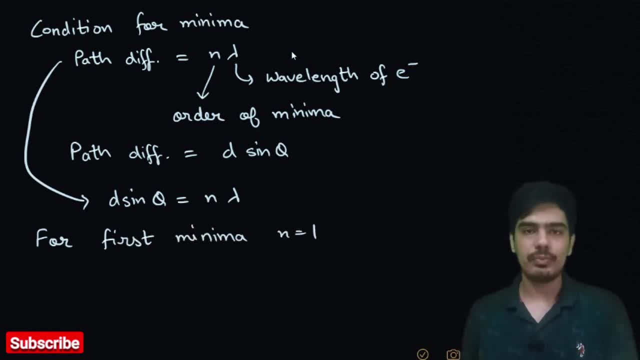 the first minima. So our n is equal to 1.. So our equation becomes: d sine theta equal to lambda. From here we can say that d is equal to lambda by sine theta, and also our uncertainty in the position of electron is equal to d. 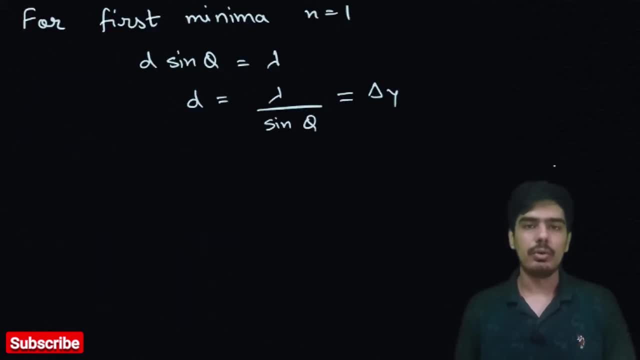 So we can replace d by delta y. So here we get. delta y is equal to lambda by sine theta means our uncertainty in the position of the electron is equal to lambda by sine theta. So now let's find out the uncertainty in the momentum. 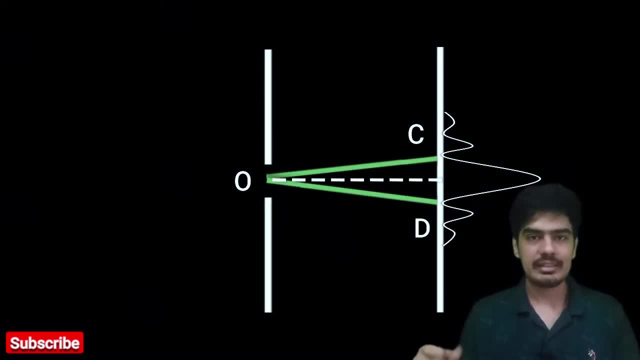 So for that consider two points: One c- This is the same point- and second, point d, which is point of minima on the other side of the central maxima. So now take p1 and p2 as the momentum vector corresponding to path oc and od. 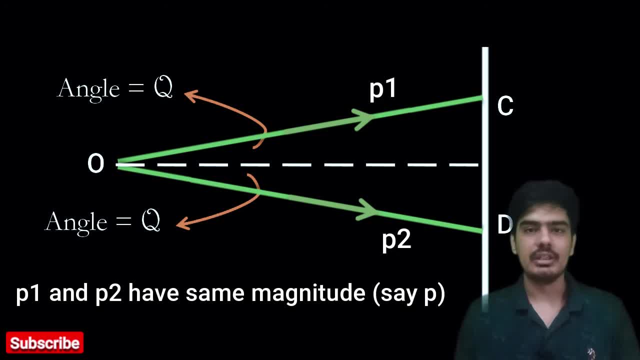 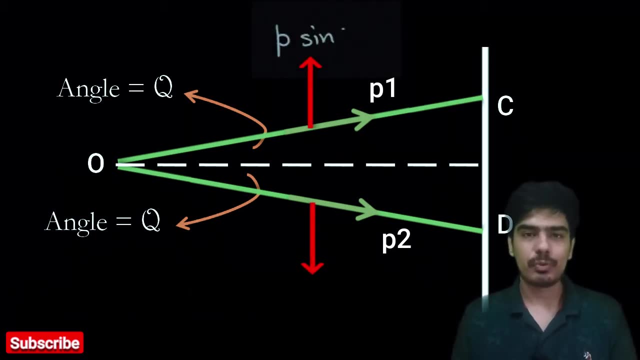 Both momentum vectors have same magnitude but different direction. So divide this momentum vector into components Along x-axis And y-axis, So our py corresponding to path oc becomes p sine theta And py corresponding to path od becomes p sine minus theta, as we have theta in opposite. 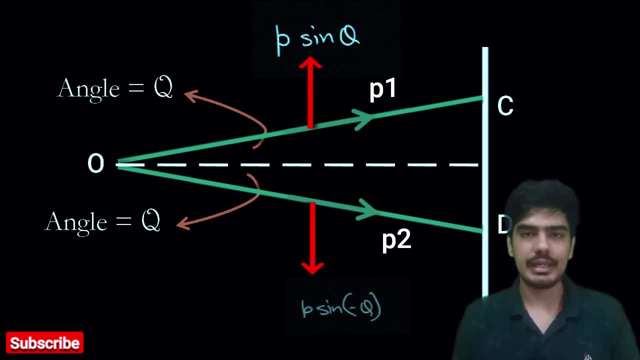 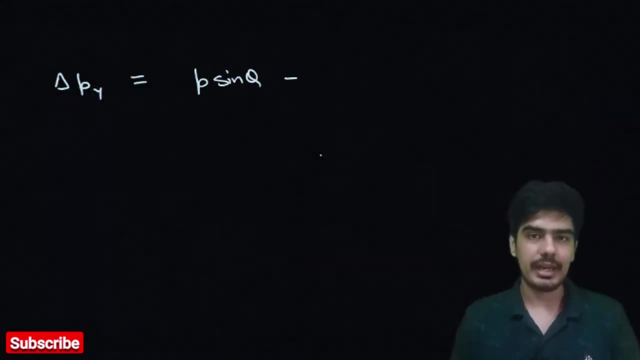 direction. So as a convention we have used negative sign here. So py corresponding to od becomes minus p sine theta. Now we have to find out the uncertainty. So for that we have to subtract these two values. So after subtracting these two values we get 2p sine theta. 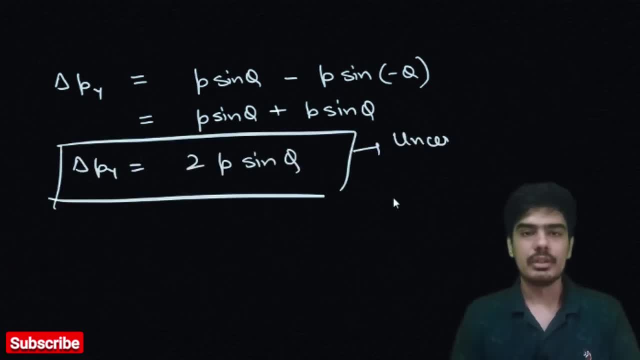 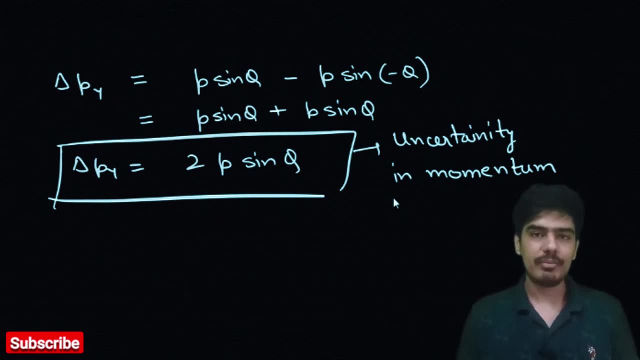 So this term represents our uncertainty in the momentum. So now we have find out the uncertainty in the position and the momentum, So let's multiply both of these. So after multiplying these two delta x and delta p, we get lambda by sine theta multiplied. 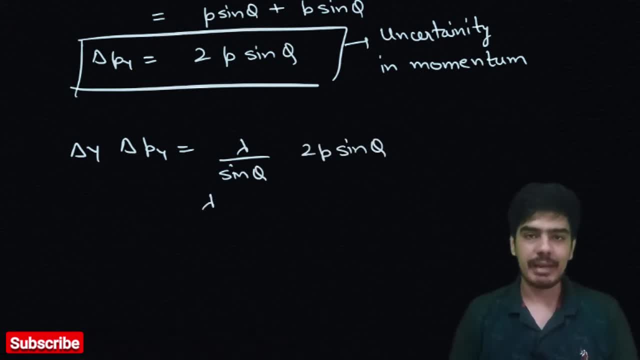 with 2p sine theta And we can substitute lambda as h by p And as a result of this, we get delta x And as a result of this we get delta x plus delta. py is equal to 2h. Now we can replace h by 2pi, h cut. 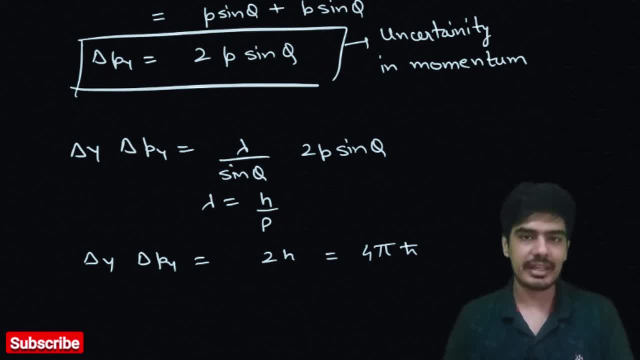 So we get 4pi h cut. So here we are observing that this value is greater than h cut by 2.. So now we have shown that the uncertainty principle is valid here. Now let's see how the width of the central maxima changes when we change the slit width. 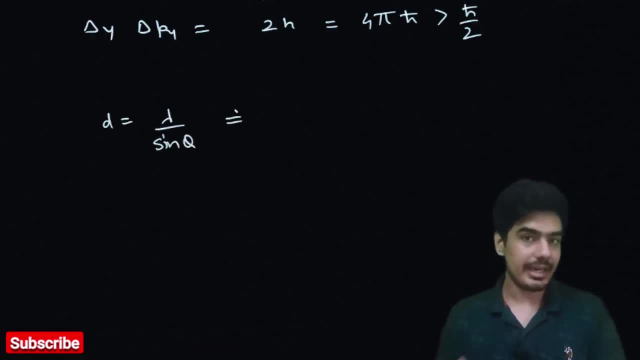 So for this you need to understand that the slit width is lambda by sine theta. That means sine theta is inversely proportional to slit width. Or you can say: uncertainty in y position of the electron And the uncertainty of momentum is directly proportional to sine theta. 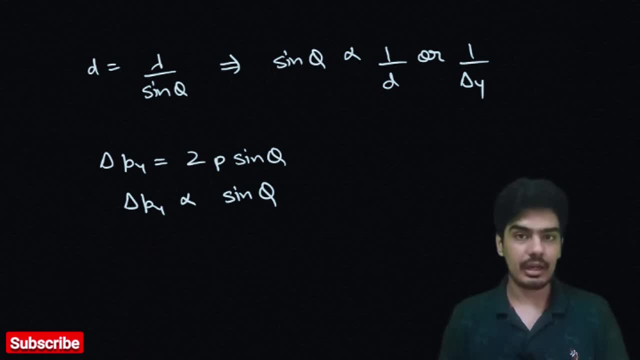 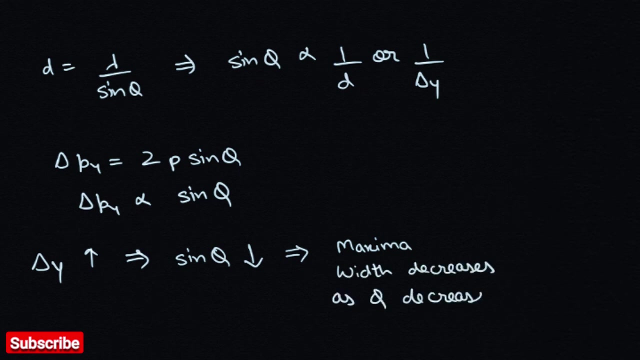 So with increase in the uncertainty along the y axis, that means increase in the width of the slit, decreases the value of sine theta. That means uncertainty in the momentum of the electron decreases. And similarly, when the slit width decreases, the value of sine theta increases. 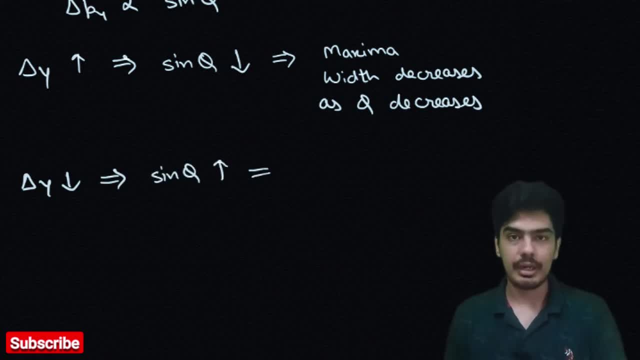 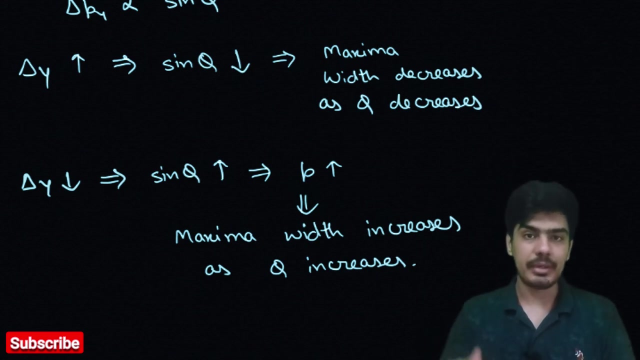 That means width of the central maxima increases. This is weird, right, That when we decrease the slit width, the width of the central maxima increases. Now I hope that you are correlating this with the uncertainty principle That when we make one thing more certain, then the another thing becomes more uncertain.